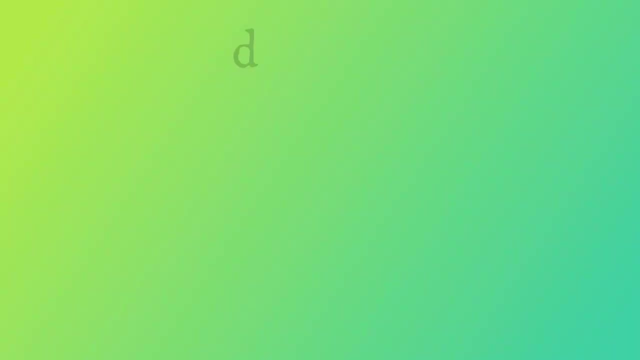 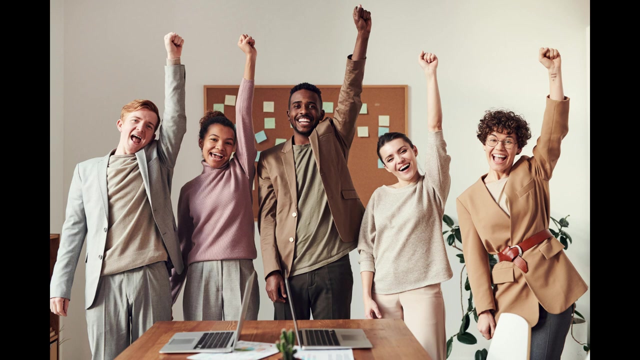 The woman on the right is wearing glasses. Focus on the details In front of the people. there is a desk. On the desk there are two notebooks, some papers and a plant. In the background I can see a notice board. Behind the woman on the right there is another plant. 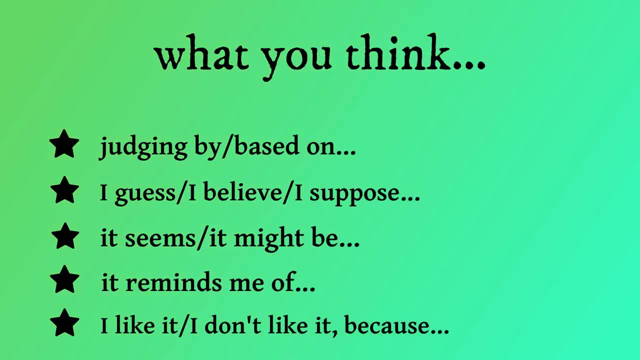 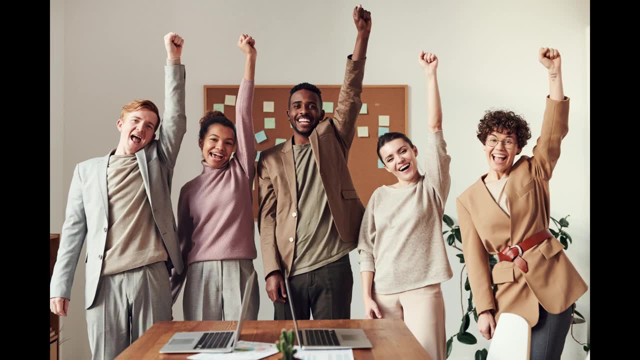 What do you think? Based on the fact that they are smiling, I believe that they like their job, or maybe one of them has just told a joke and that's why everybody looks so happy. I guess they are good friends and that they like each other. 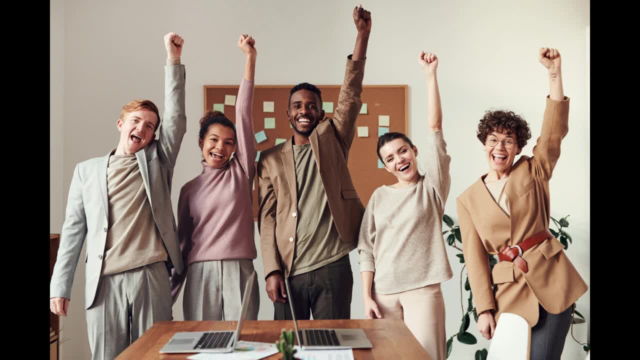 Because of the clothes that the people are wearing, I think it's Friday. Their clothes are not entirely formal and many offices have casual Fridays, which allows their employees to dress casually. I like this picture because everybody in it is very relaxed and they seem to be a good team. 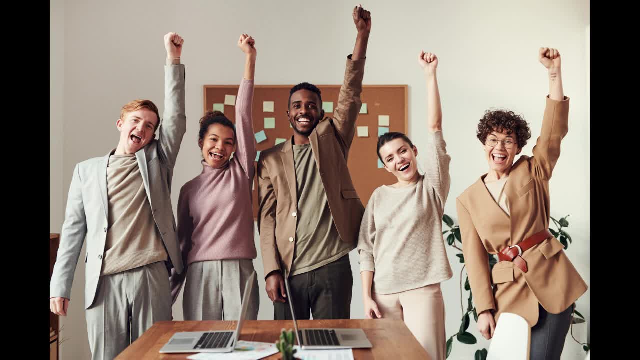 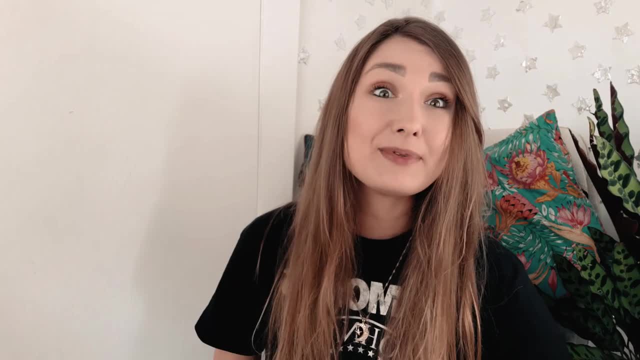 It reminds me of my parents' office, where the people are very friendly and helpful, and I think I'd like to have colleagues like that in the future. And now I will describe two more pictures for you. In the picture I can see two boys. 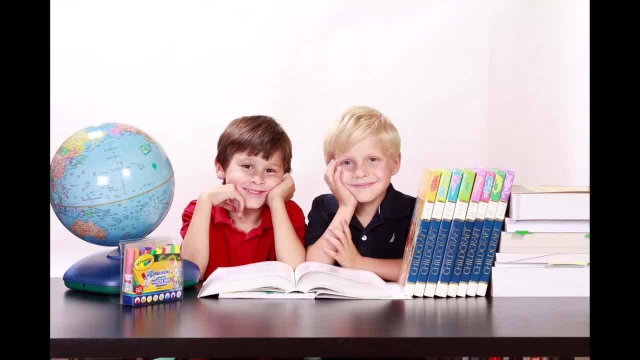 I guess they are both six or seven years old. On the left side of the picture there is a globe and on the right side of the picture there are some books. The boys are in the middle of the picture. They are both sitting and smiling. 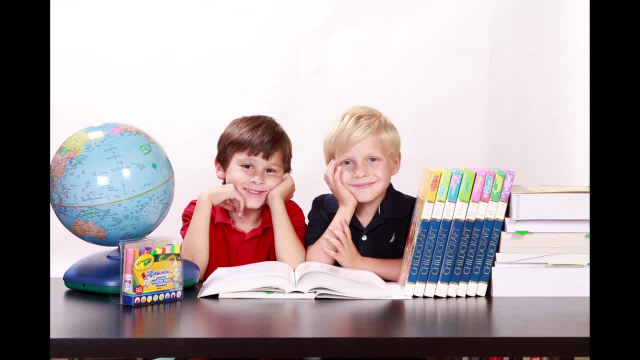 The boy on the left is wearing a red t-shirt and the boy on the right is wearing a black t-shirt. They are sitting next to each other and they are reading a book. I believe this is a geography book because of the globe that is standing next to the boys. 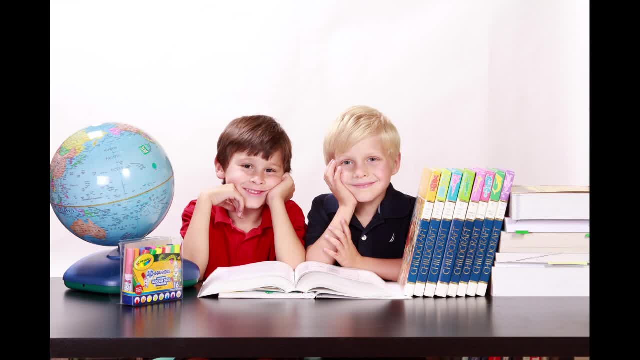 Judging by the fact that there are a lot of books and no toys in the picture, I think the boys are at school. It seems that they like it because they look quite happy. I guess they are best friends and that's why they are sitting together. 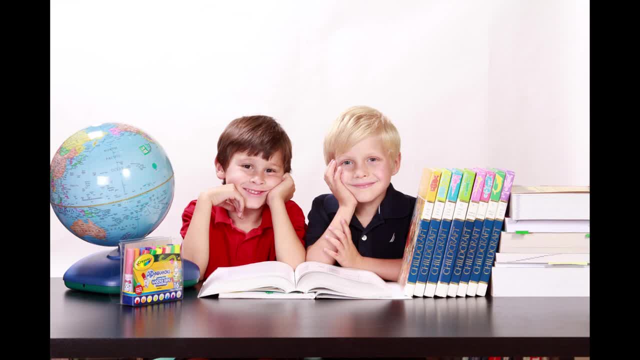 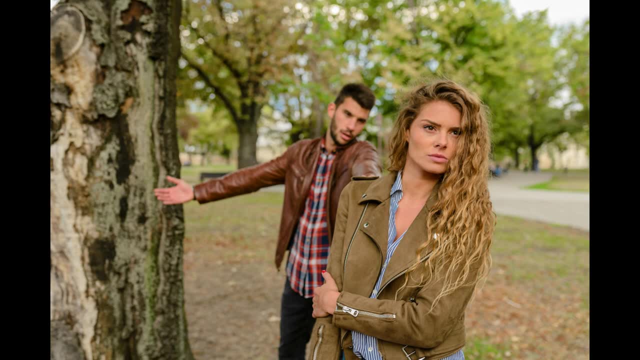 It reminds me of my school friends and how we used to learn and play together. In the picture I can see a couple, a man and a woman. They are in the foreground and in the background there are some trees. There is also a really big tree on the left side of the picture.